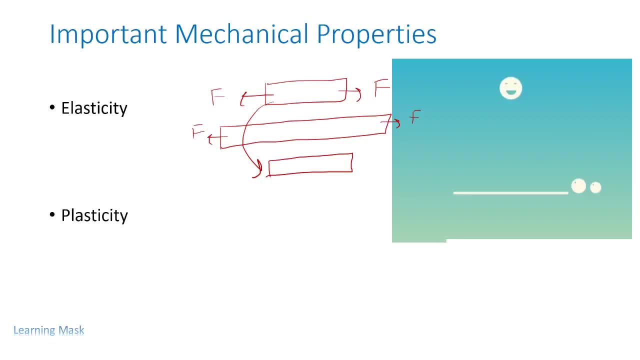 Now, next property is plasticity. Suppose we have a object, This is our object, and if I am applying force and it get deformed after application of force, When I remove force from this material, then the material does not come back to its original position. That is this position and this position is not same. that is, it is deformed. This type of material is called plastic and the property by which it is getting deformed is known as elastic material. 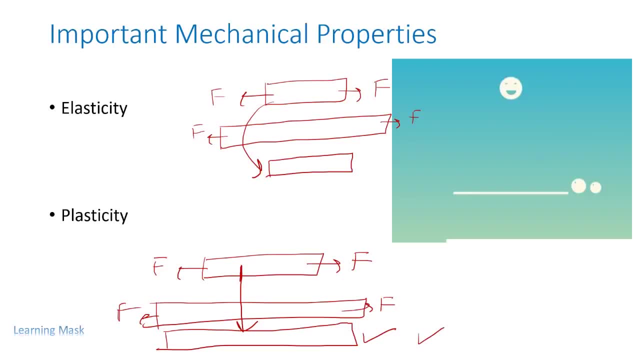 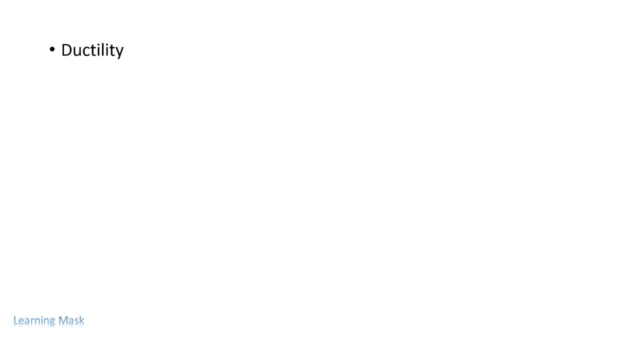 So this material is not coming form and it is not coming back to its original position, which is plasticity. Next property is ductility. Ductility mean any material. Suppose this is our material and if we can change this material into wire by application of force, 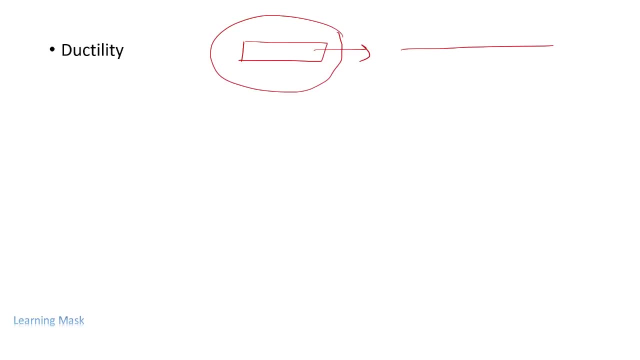 then this property called ductility. Next property is Bittleness. Suppose we have a material and by application of force or any pressure, questo material, this material breaks, that is, they cannot be changed into wired form. so this type of material is called brittle material. example of brittle: 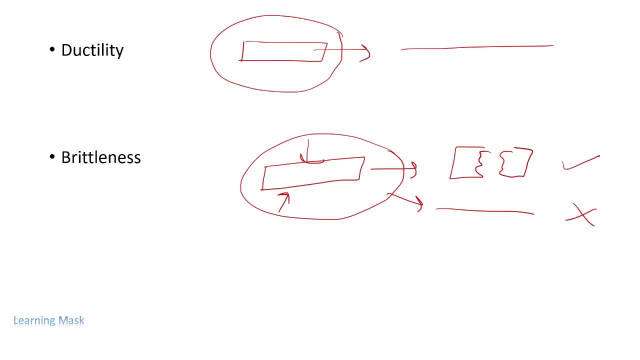 material is glass. an example of ductile material is gold, copper, wire, etc. next property is known as malleability. now, malleability is a property in which a material can be changed into thin sheets. that is, by application of pressure in all sides. we are changing this material into sheets, so this is known as. 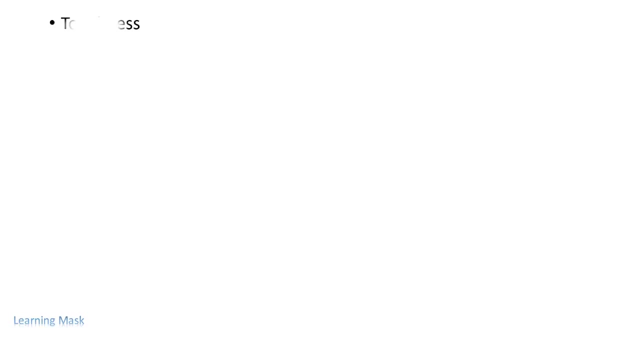 malleability. next property is toughness. toughness is defined as property of a material which enable it to absorb energy without fracture. suppose this is our material and if a force is applied in this and the energy absorbed by this material becomes a material which is called malleability, and this material is 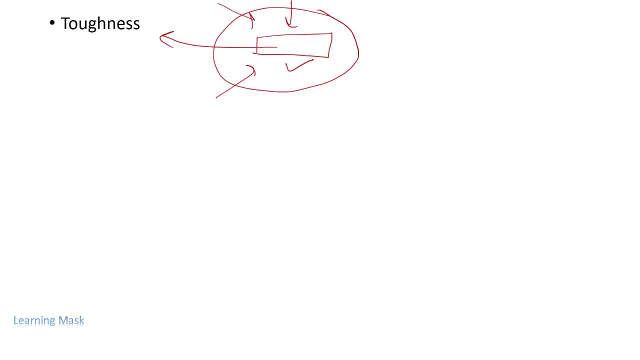 before, fracture is known as toughness. now let's understand this with a graph. suppose I am drawing graph between load, that is P, and elongation, that is Dell, TL is our elastic limit and F is our fracture point. so suppose this is our material and if I am applying any type of load, say I am applying load P and 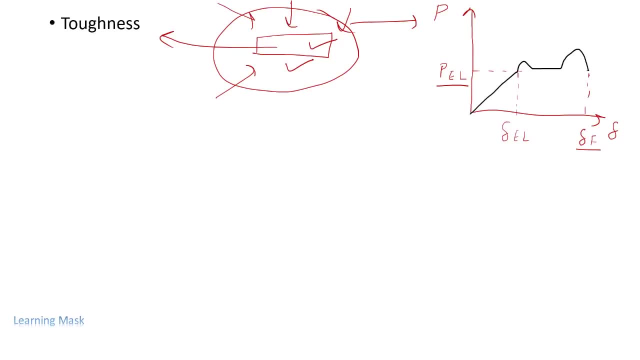 after application of load. this is fracture point of the material means after this point the material get fractured. So the energy absorbed by material till this point is known as toughness. Next we will discuss hardness. Hardness is ability of a material to resist indentation or surface abrasion. 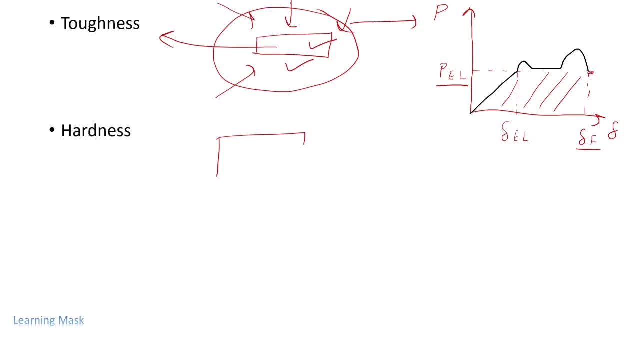 Let's understand this. Suppose we have a material and if I am applying any type of load in it, so there is no surface cracks, there is no indentation in this material and there is no abrasion in this material. That is suppose this is our material and if I am leaving a heavy ball to fall in this material? 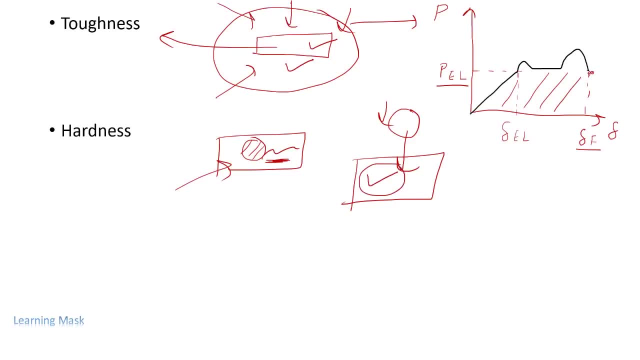 then there will be no depression form here, there will be no cracks in this material. If no crack is formed, then this material is hard material. So hardness is the ability of a material to resist surface abrasion, to resist cracks, to resist indentation. 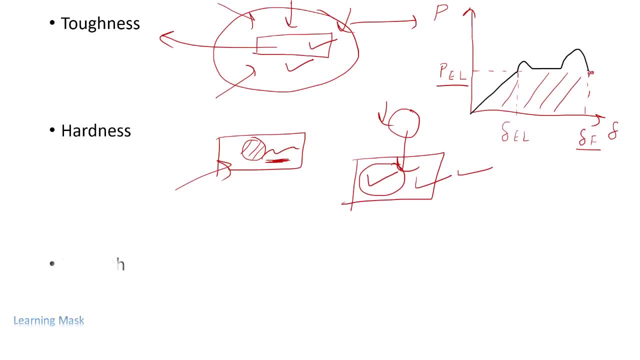 Next problem, The property which we will discuss is strength. Suppose we have a material and if I am applying a force, say a compressive force, and if the internal resisting force are developed, if we apply force in a material, then internal resisting forces are developed. 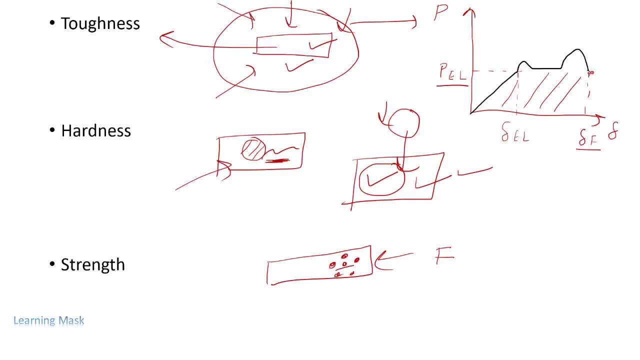 Then this force? they generally resist the deformation. If I will apply force in this material- suppose this is our material- if I apply force, then this material should deform like. this means it should deform like this. But what is happening? internal resisting forces are developing and it is resisting. 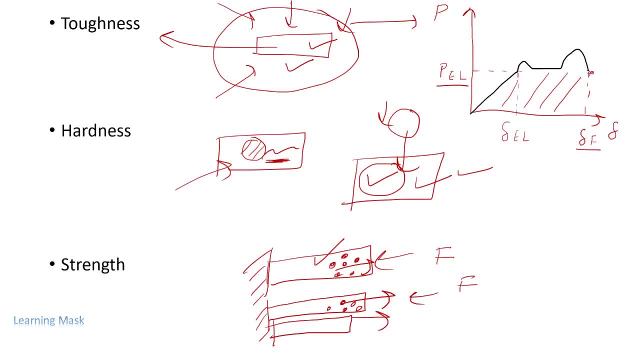 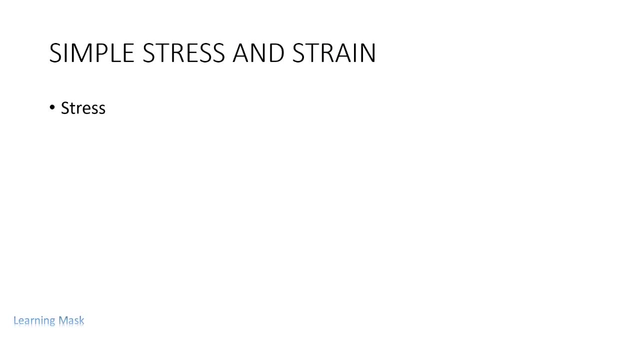 this force in opposite direction. in this direction, Then this internal resisting force is known as strength of that material. Here we will talk about simple stress and strain. First let's define what stress means. Suppose we have a material and it is subjected to a force F. 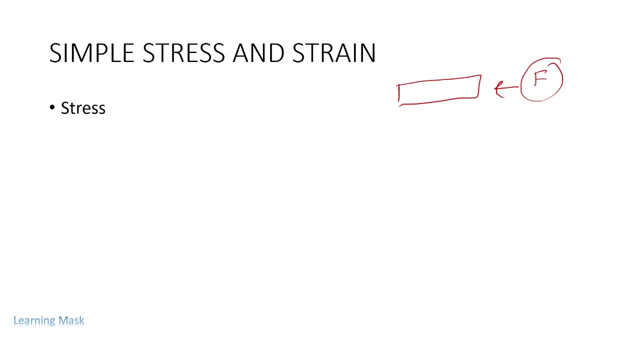 This is our external force. When an external force acts on this object, then a resisting force is set up within the component. So these are resisting forces which act this side. So the internal resistance force per unit area acting on material is called stress. 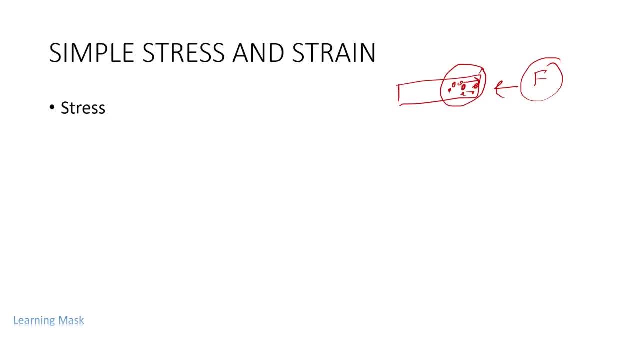 So these internal forces, divided by area, is known as stress and it is having unit as Newton per meter square. Now we will classify stress, Stress, Stress, Stress, Stress. So we classify stress as simple or direct stress, indirect stress or combined stress. 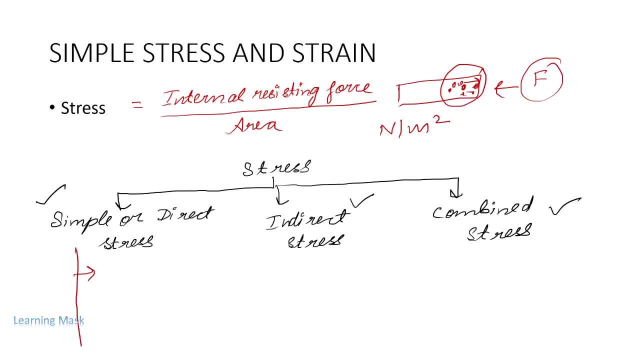 And in simple and direct stress we have three classifications: First is tension, which we can say tensile force, Second one is compression or compressive force, And third one is shear. When we talk about indirect stress, then we have two categories. 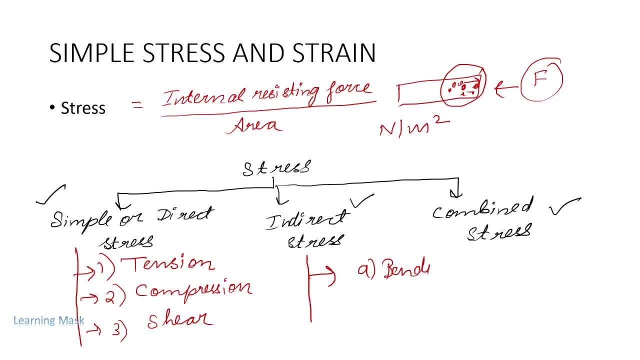 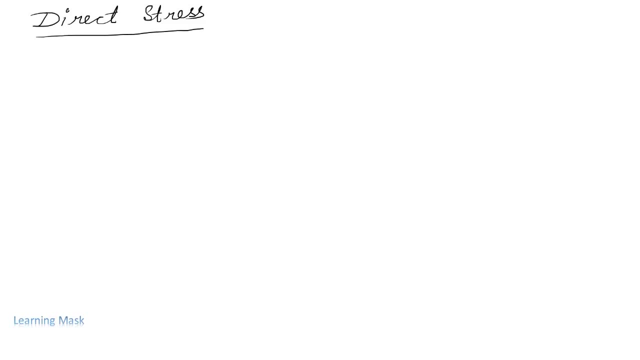 One is our bending, and second classification is torsion. Now we will understand direct stress. If a force acts on an object directly, that is, if force acts normal to the cross-sectional area, then that force is known as direct force and that force will develop a stress which 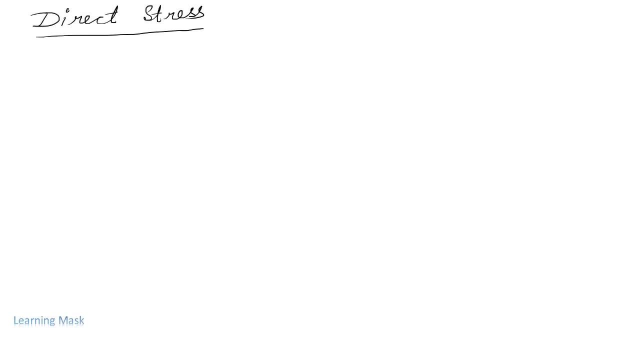 will be direct stress. So let's understand direct stress. Let's understand this with an example. So you can observe in this image that force is applied directly to this surface. If you will see this cross-section, then this cross-section is this: and force is acting. 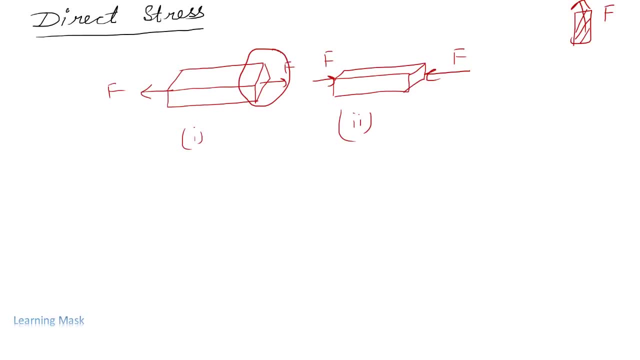 perpendicular to it. So this force will develop a stress which is direct stress. So we will define direct stress as ratio of force to area. Now you can observe here: the tendency of this force is to elongate This surface. So tendency of this force is to elongate this surface. 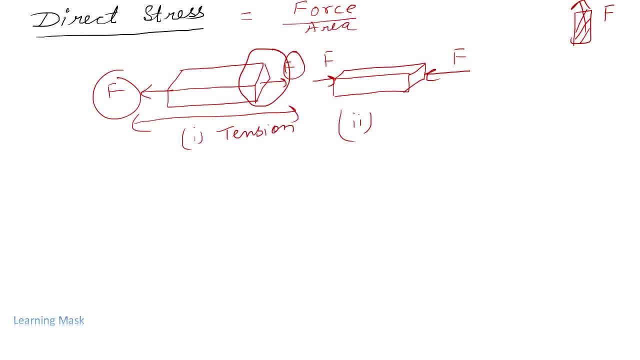 So this force is known as tension, And if you will observe this force, then this is compressing. this object means it will shorten the object. So this object force is known as compressive force, that is compression. Now we will talk about third case, which is called shear. 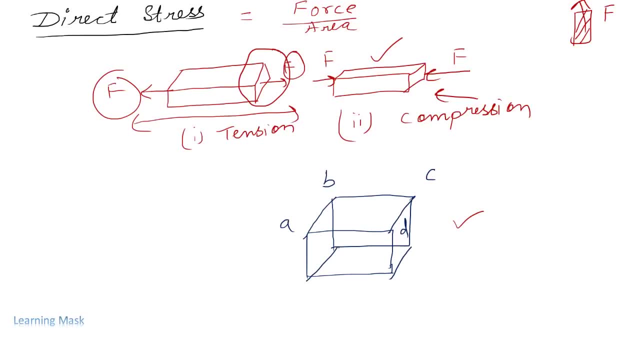 Suppose this is our surface And if force acts parallel to the cross-section area, then these force will develop a stress which is known as shear stress, And the force which acts parallel to surface is known as shear force, and they will develop shear stress. 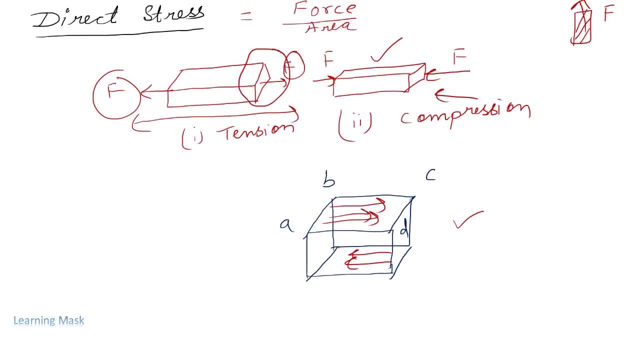 So we can define shear stress as shear force per unit area. So we use this symbol, tau, And this is our force. This is our force, that is shear force, and this is area of cross-section. that is this cross-section where shear force is acting. 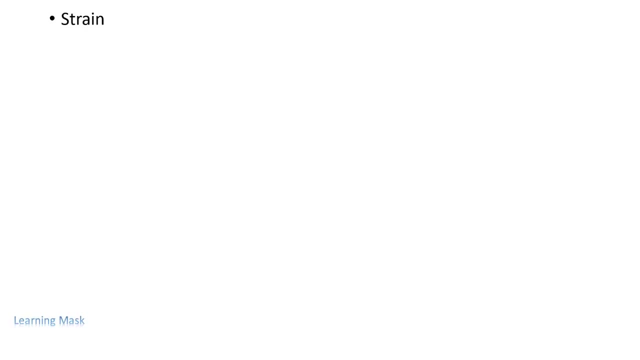 Strain is defined as ratio of change in length to initial length. So let's see what this means. This is our surface in which a force, F, is applied. This is length, and suppose T is our width. So if we apply this force, so this force will elongate the surface, it will elongate the 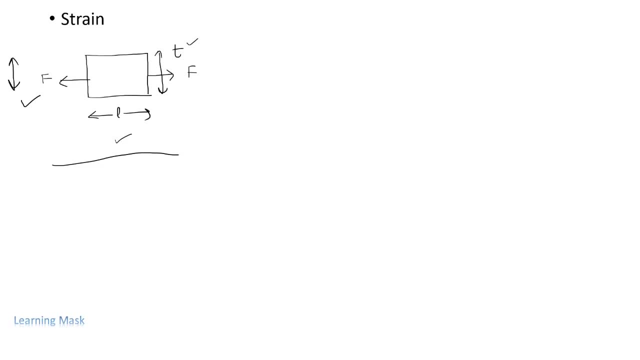 surface. It will decrease this T. that is our width, So it will look like: So del L is our increase in length. So this is del L and this is our decreased width. that is del T. both side here also del T. So now we will define two type of strain. 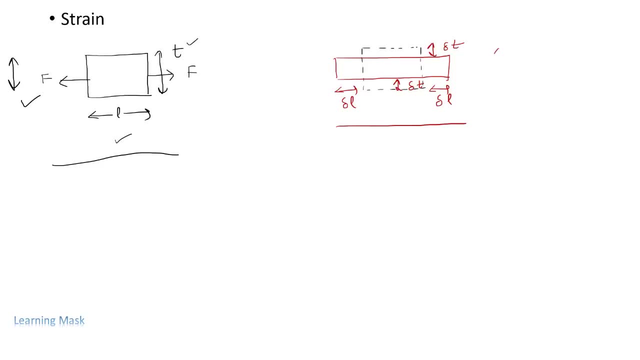 One is linear strain, that is this side strain, and one is lateral strain, that is this reduced cross-section. So we define strain as change in length by initial length. So both side length is changing, that is, here it is increasing and here it is decreasing. 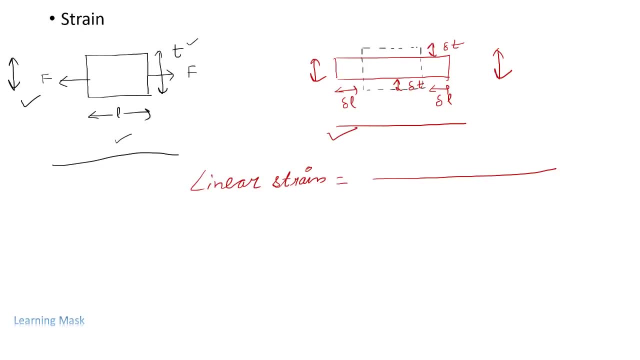 So we define linear strain as ratio of change in length by initial length. This is our linear strain. We can directly put this value in it. That is, our initial length is L and change in length is del L plus del L. Now we will define lateral strain. 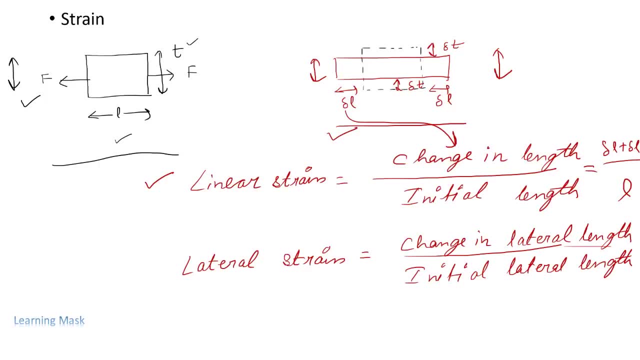 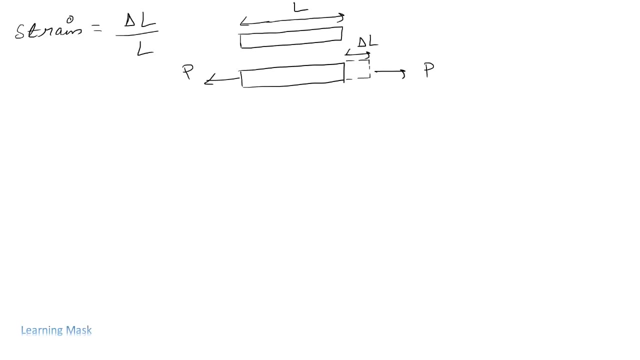 So similarly we can say: it is change in lateral length to initial lateral length, that is, ratio of change in lateral length to initial lateral length. that is del T. So this is how we define strain. Now we define mathematically strain as ratio of change in length to initial length. 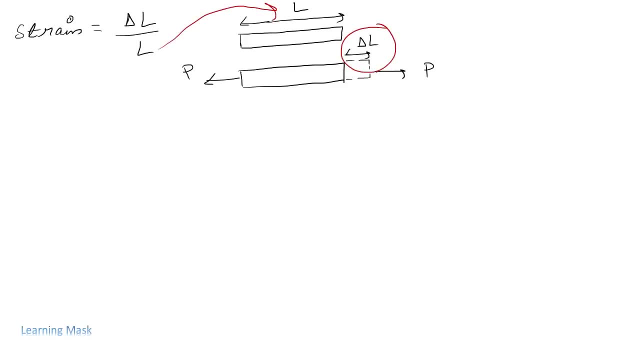 So this is our change in length and this is our original length. Now we will define shear strain. So So this is our object and this is our shear force, that is, force which is acting tangentially to our surface. Now, when this force act to this surface, then this layer will slide forward. so it will look. 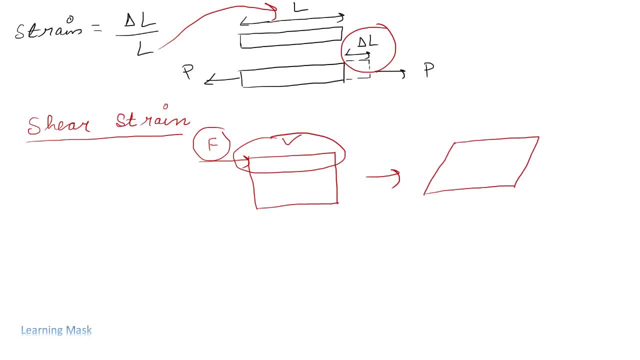 like. So it look like this. That is after application of force. this upper surface has slided, So I have combined the figure. So del L is our displaced length of the side And phi is our angle strain angle. So we define shear strain as phi. 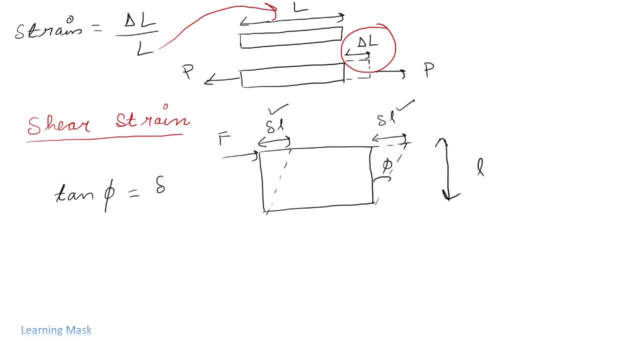 So phi is our shear strain, So we write tan phi as del, L by L. So L is our this length and del is this, del is this length as shown. So we write shear strain as del, L by L, for, as we know, for small angle tan phi is equal. 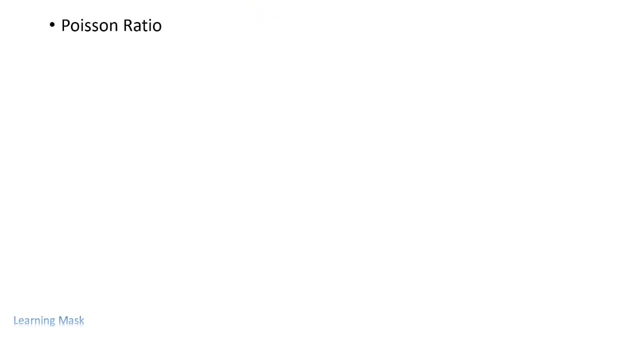 to phi. So this is our shear strain. Now This is our Poisson ratio. it is defined as ratio of lateral strain to longitudinal strain And it is denoted by symbol mu or 1 by m. So we write it mathematically as negative of lateral strain to longitudinal strain. 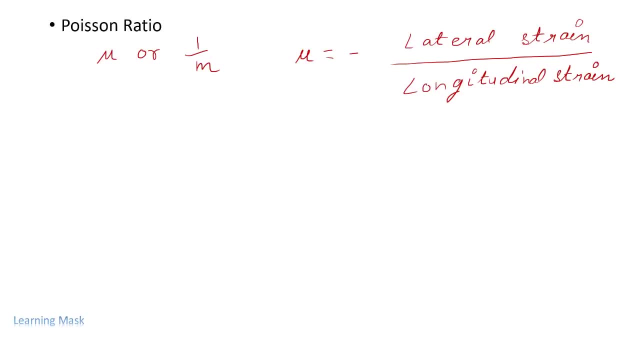 As ratio cannot be negative. So lateral strain and longitudinal strain should be of opposite sign. Just remember the figure That we have shown you in strain, So I will use same figure for finding out value of Poisson ratio. So this is our figure here: del T show our lateral side and del L is our longitudinal. 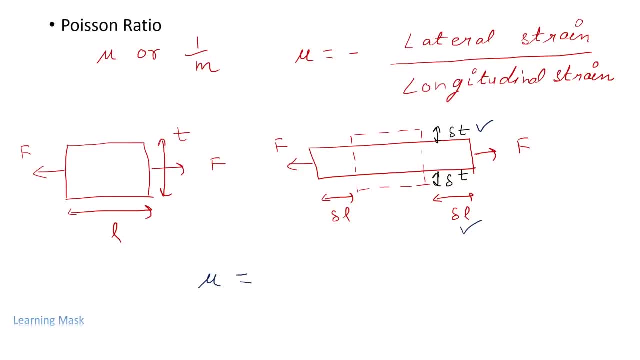 side. So we will write Poisson ratio as ratio of lateral strain to longitudinal strain. So expression is: So: this is our lateral strain, that is this strain, And this is our longitudinal strain, that is this strain. So here we have 2 del L. 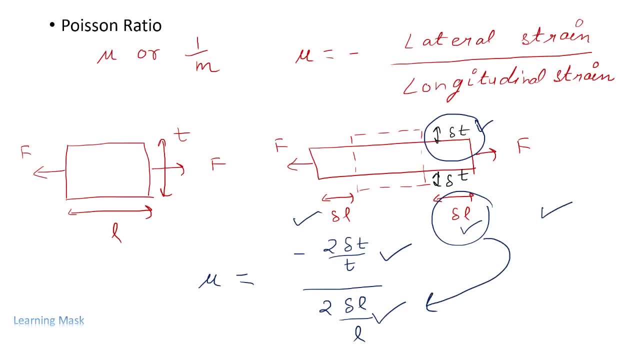 So we have added this to get 2 del L and here also we have 2 del T. So we have added this to get this. So you can also check that mu should be positive for making this positive. value of this should be negative. 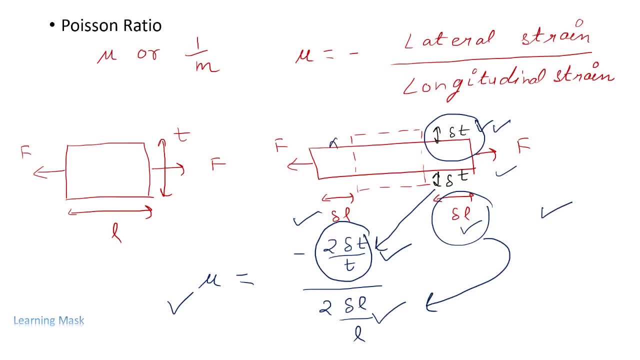 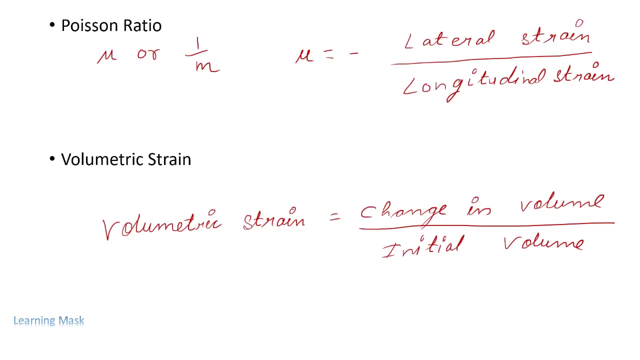 So we will put negative value, because here cross section is decreasing this side and length is increasing. So Poisson ratio is a positive quantity. Now we will define volumetric strain. So it is ratio of change in volume to initial volume. So this is how we write volumetric strain: change in volume by initial volume. 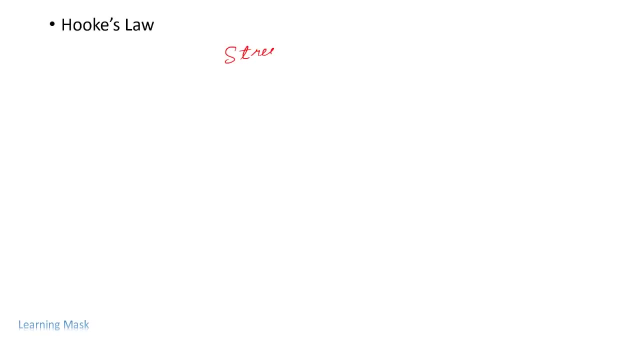 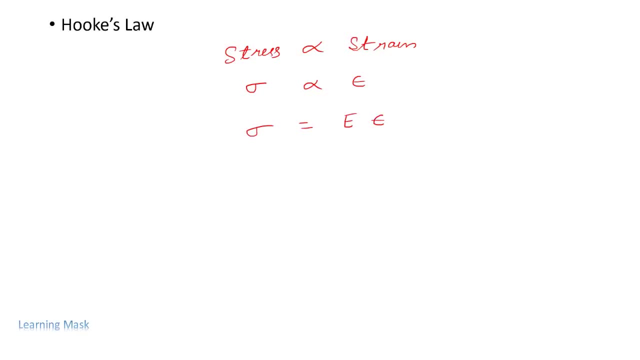 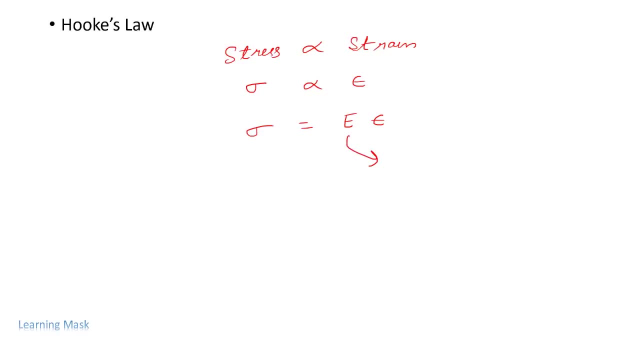 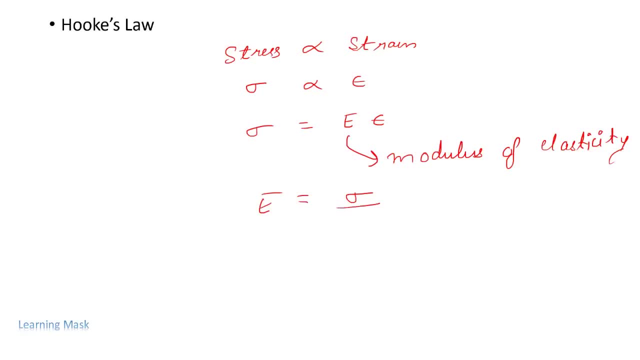 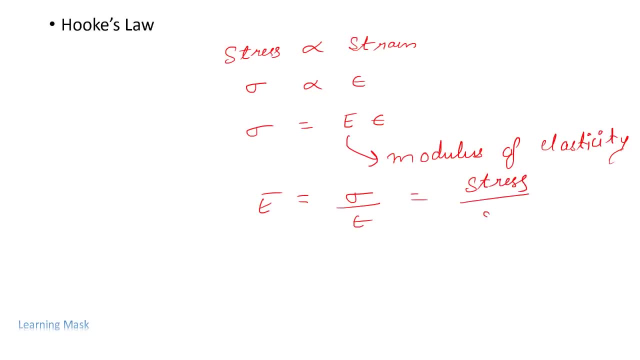 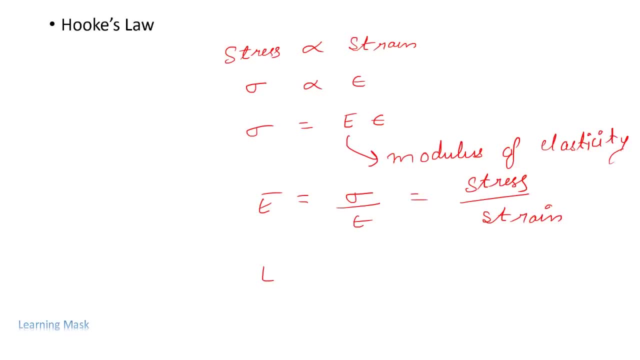 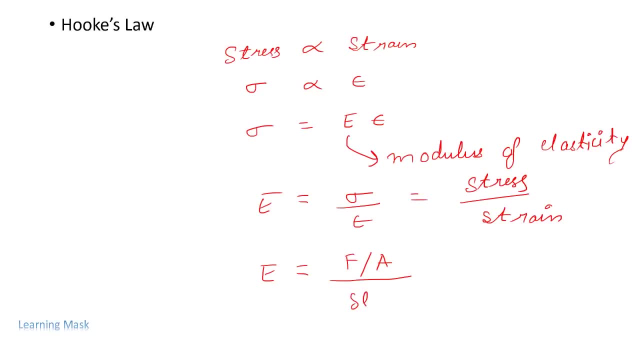 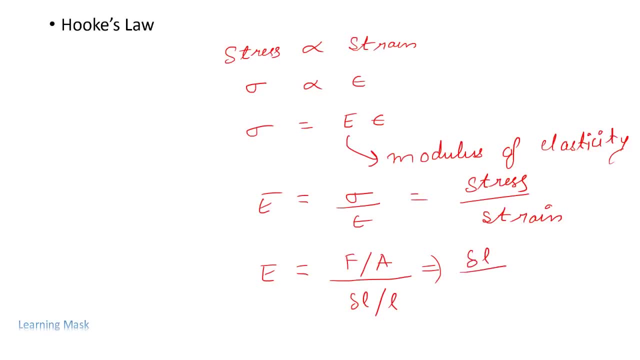 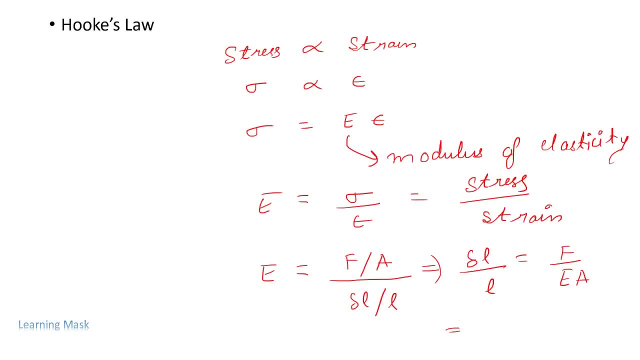 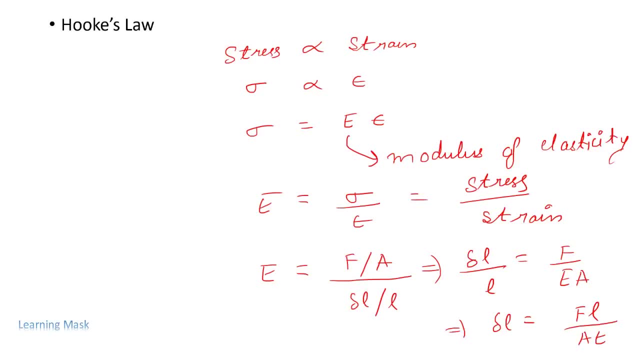 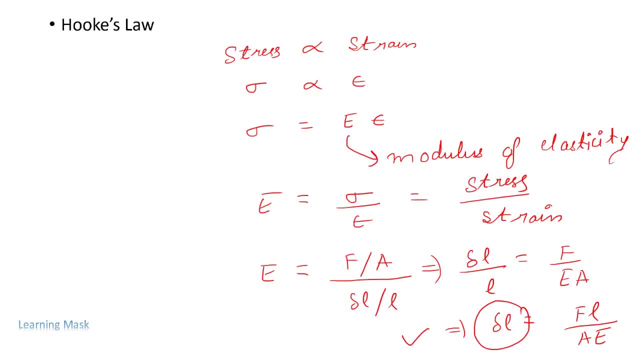 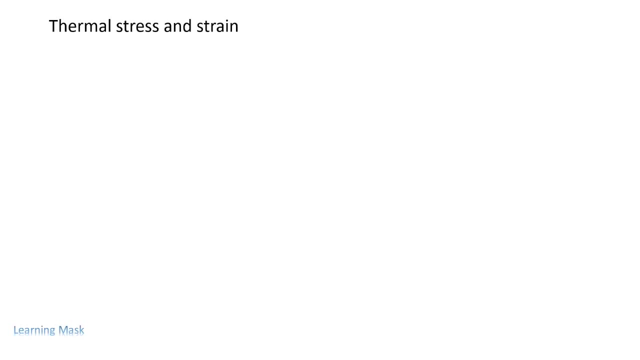 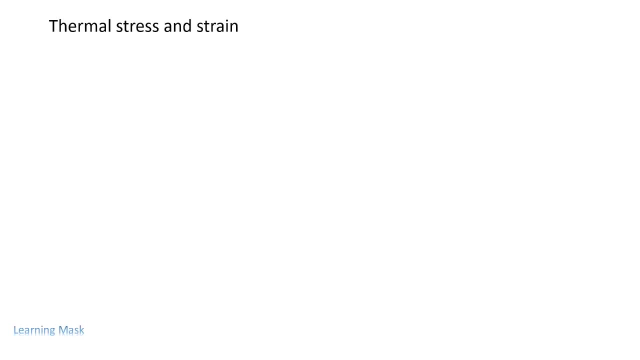 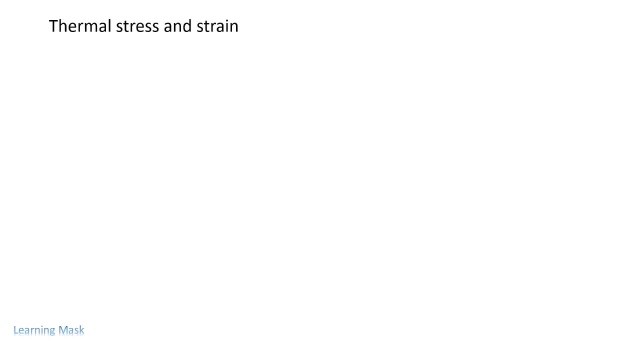 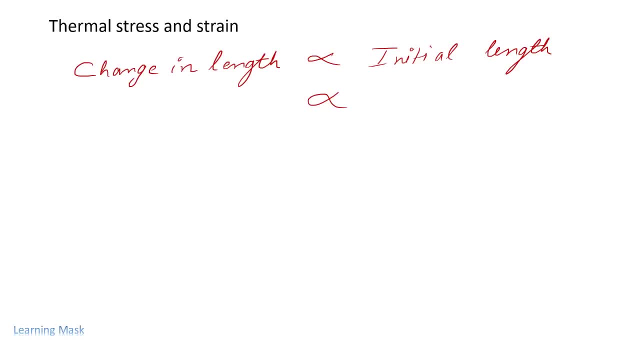 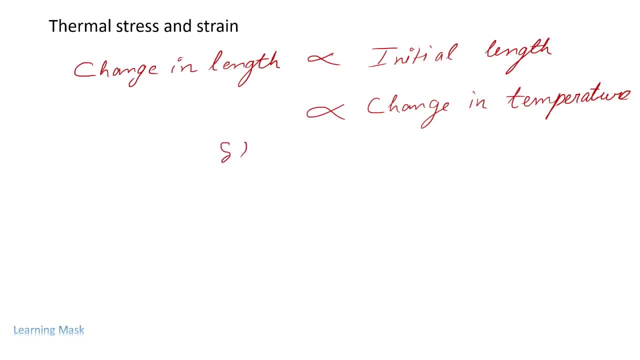 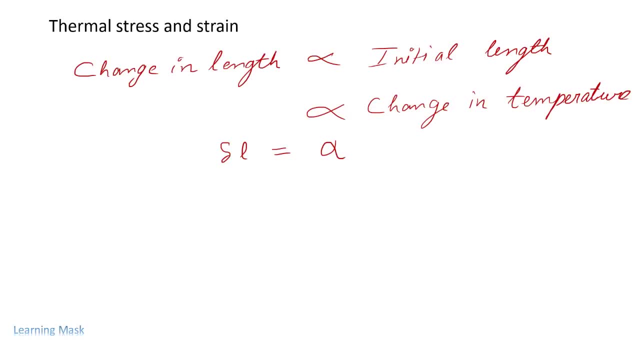 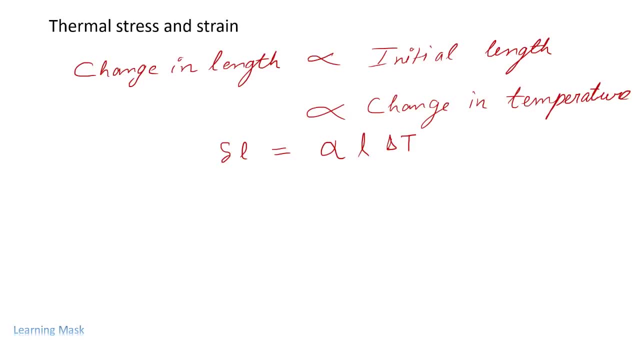 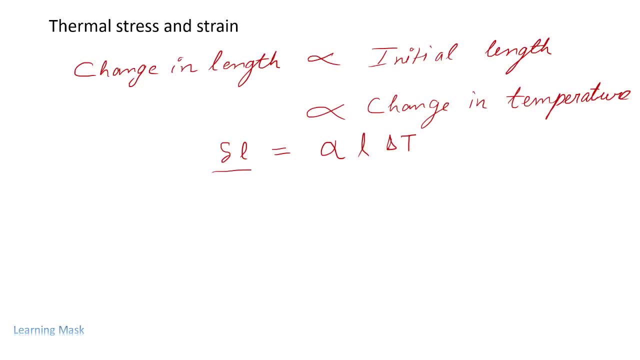 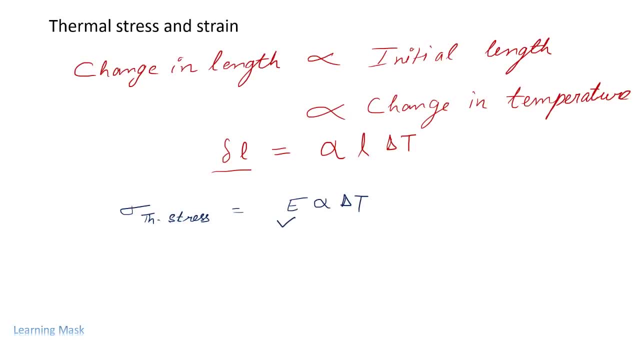 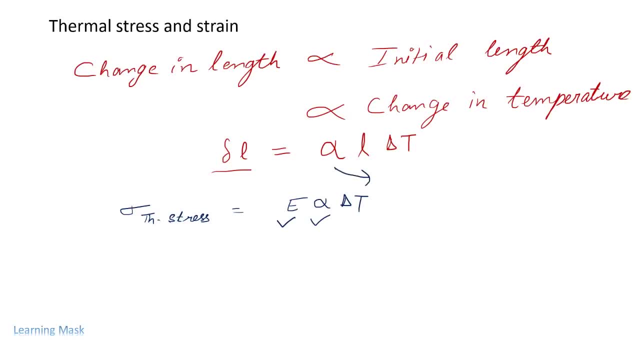 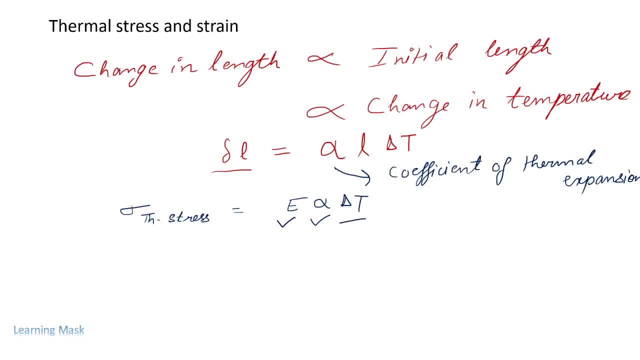 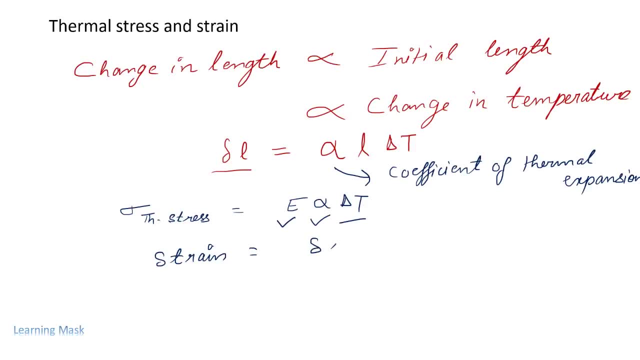 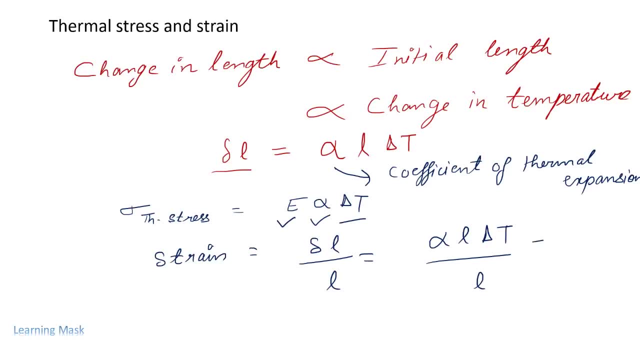 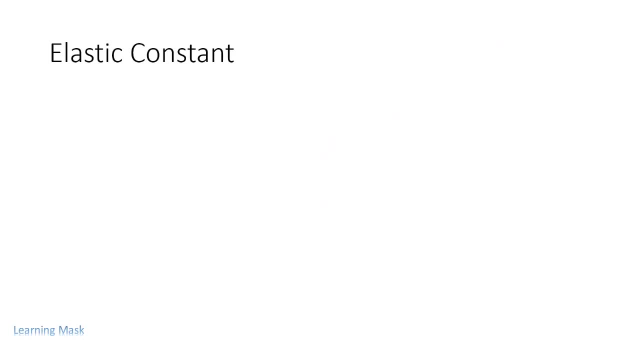 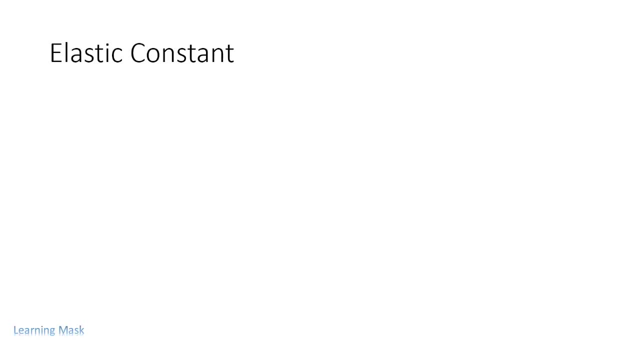 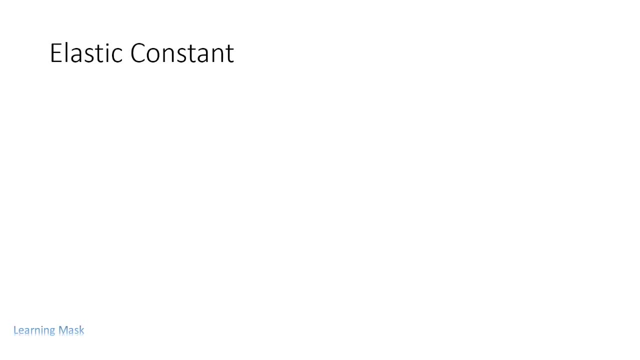 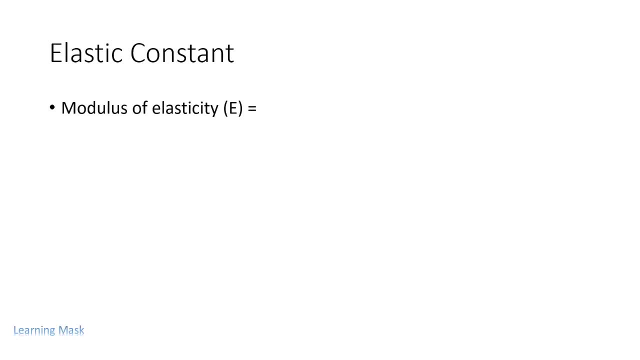 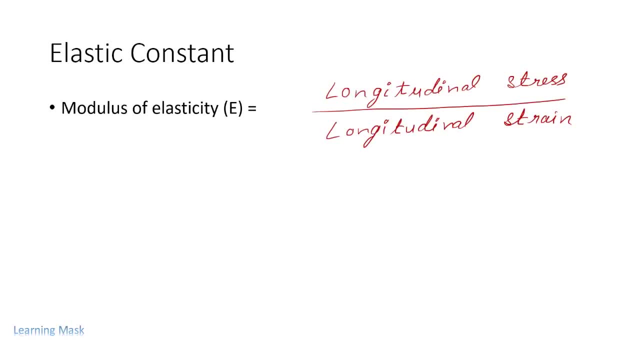 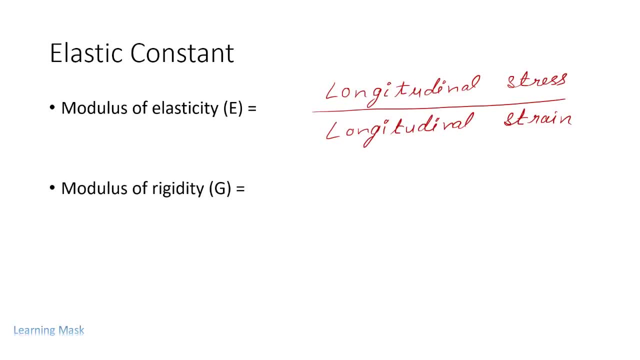 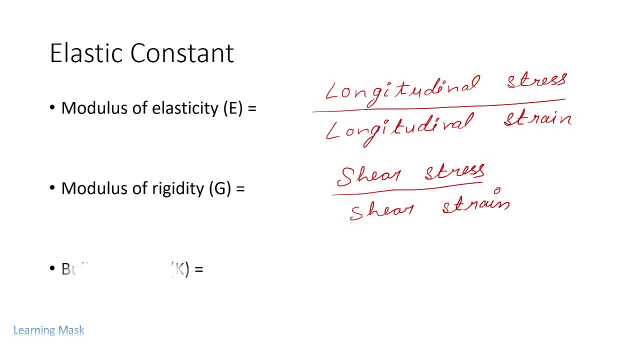 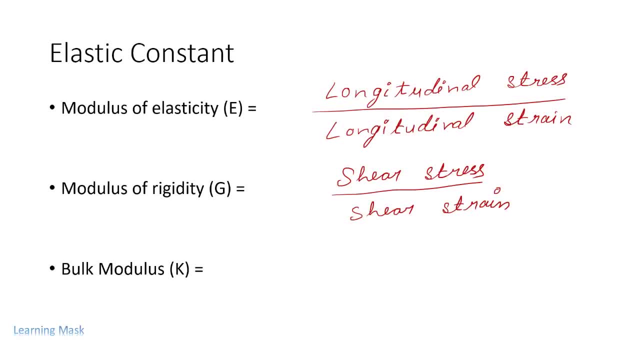 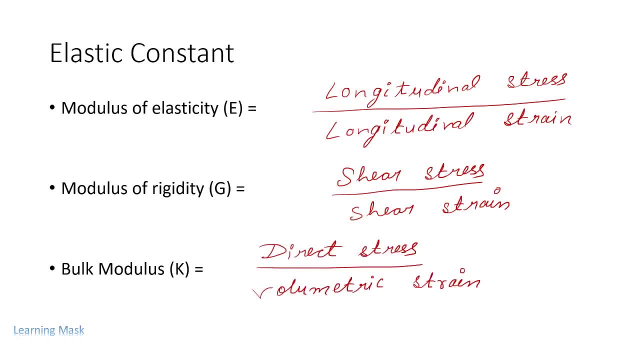 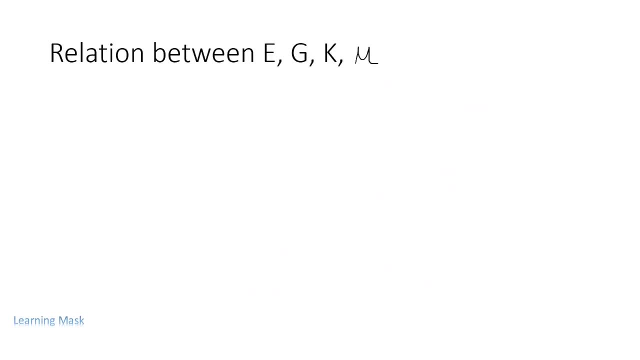 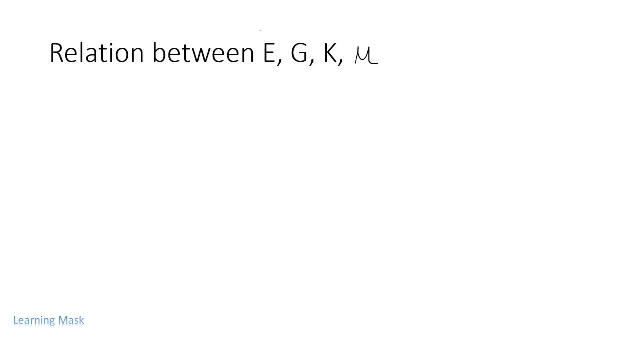 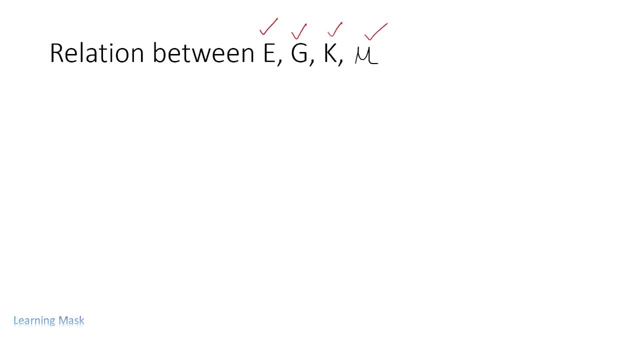 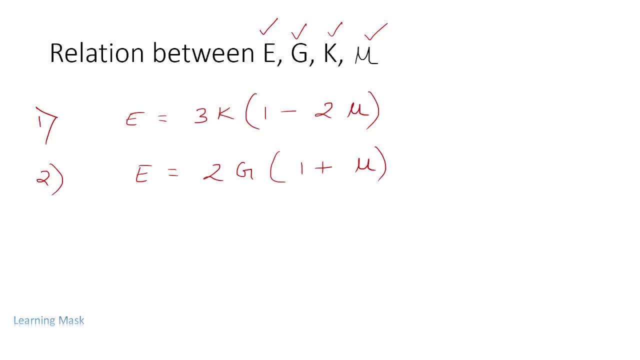 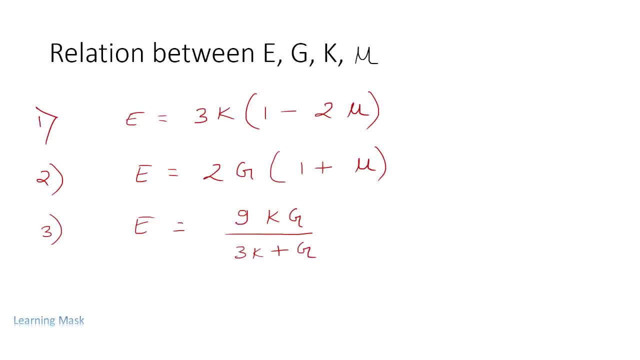 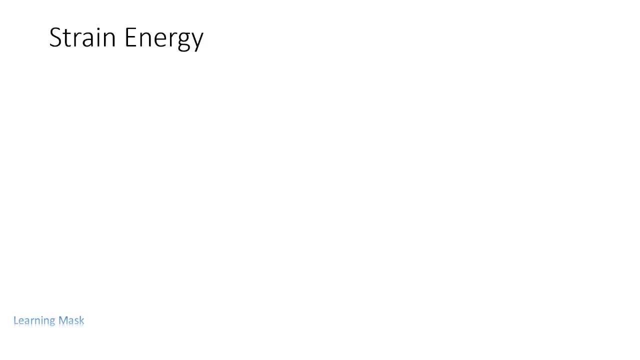 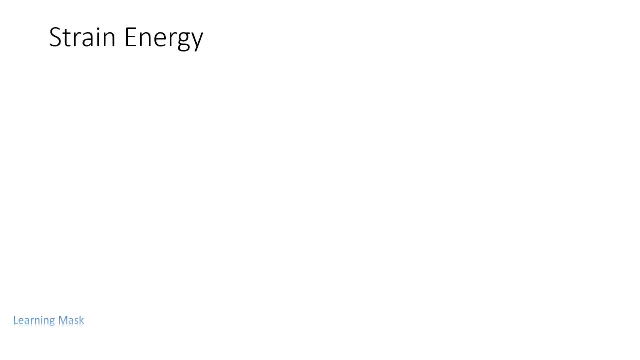 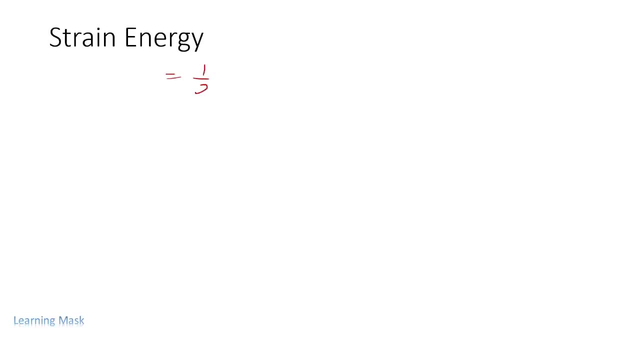 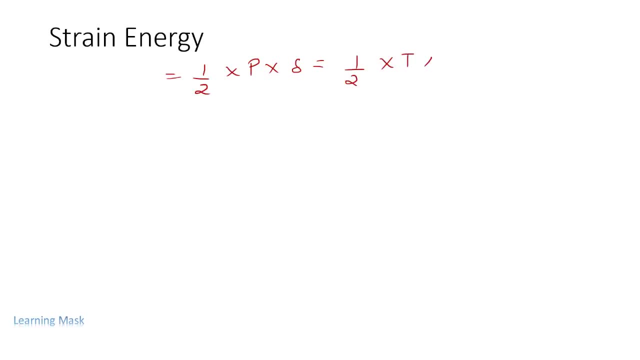 So this is strain energy mathematical expression. here P is the applied load, delta is our elongation, that is, increase in length, and T is applied torque and theta is twist by the torque. Now we will define resilience. Resilience is the ability of a material to absorb energy in the elastic region where 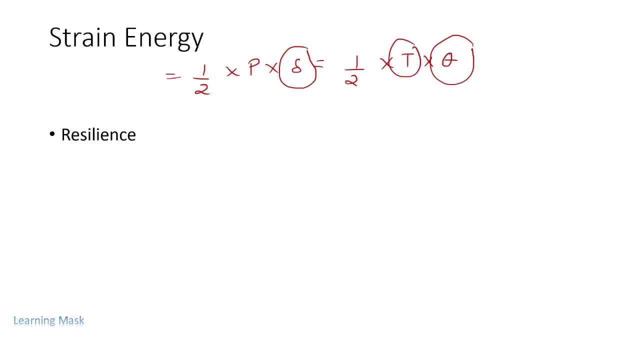 it is strained. So when we talk about strain energy, we have said that it is ability of a material to absorb energy when it is strained. but when we talk about resilience, we say ability of a material to absorb energy in the elastic region. so we are talking about elastic region here. 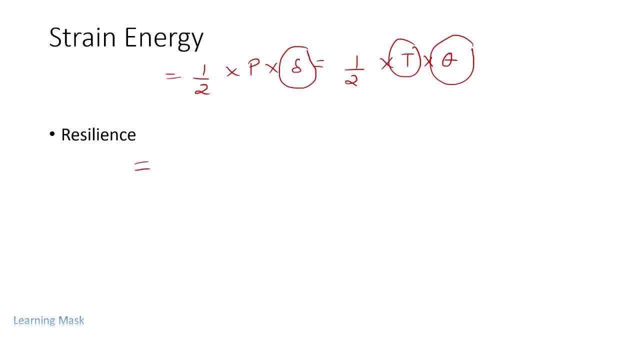 So we give this by expression: area under P, delta curve. That is half into P, into delta. so we generally talk about elastic limit here. so don't forget this elastic limit in resilience. that is elastic region. Next we will talk about proof resilience.